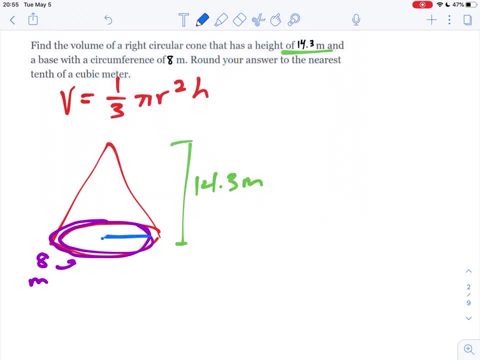 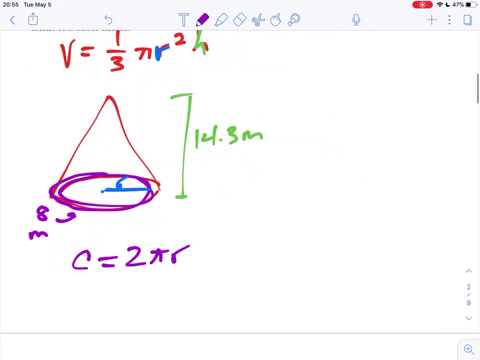 a radius which is this length here from the middle to the edge. So we need the radius which we don't have. So a prerequisite to this problem is to find the radius. and hidden within the circumference is the radius, because the formula for circumference is 2 pi r. 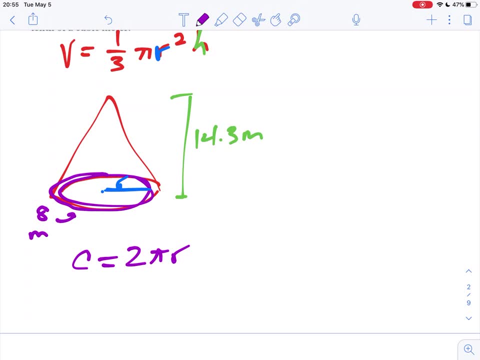 But we know that the circumference is 8, so I can say that this amount is equal to 8.. So in order to solve this for my radius, I'm going to divide both sides by 2, and this will give me pi times radius equals 4.. And then, if I divide both sides by pi, I get 4. 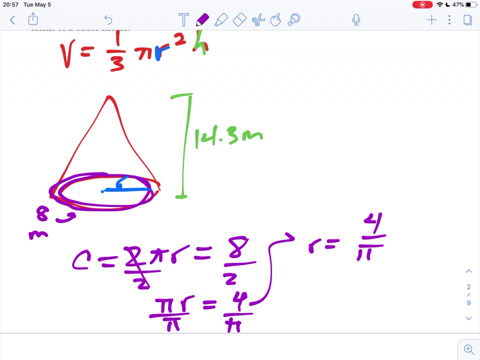 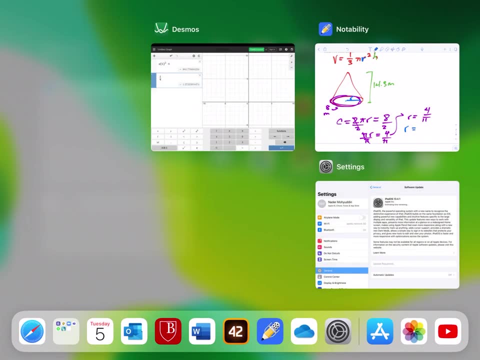 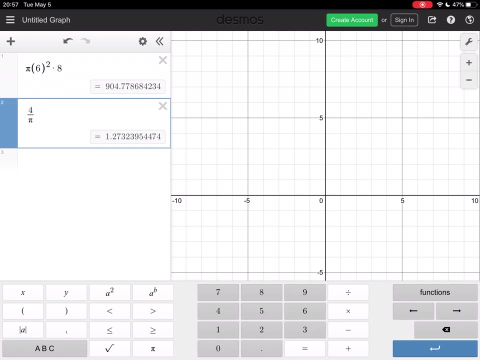 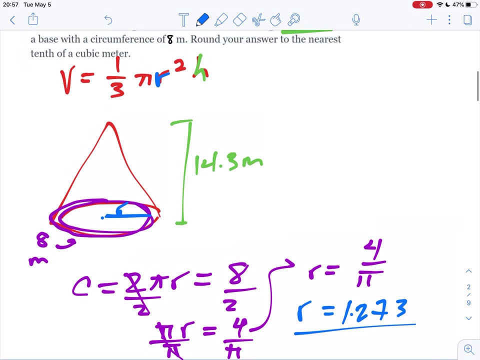 divided by pi. I can divide by pi, here and here, mathematically, And what you'll find is that the radius 4 divided by pi is 1.273.. 1.273.. Okay, crisis averted, We now have the radius. We already had the height, so now all we're. 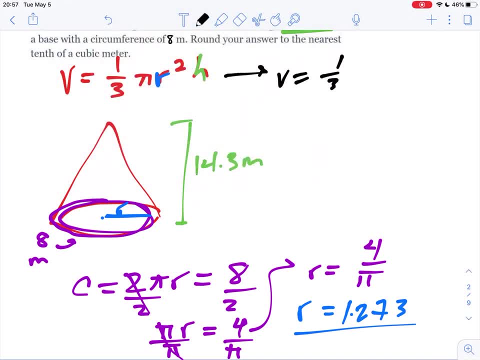 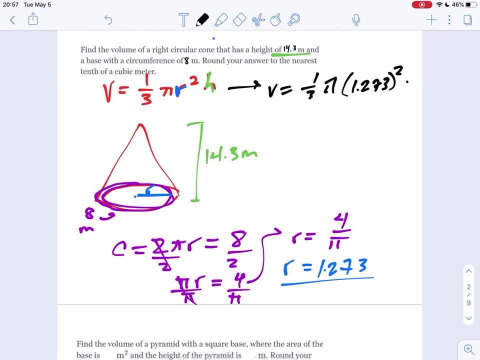 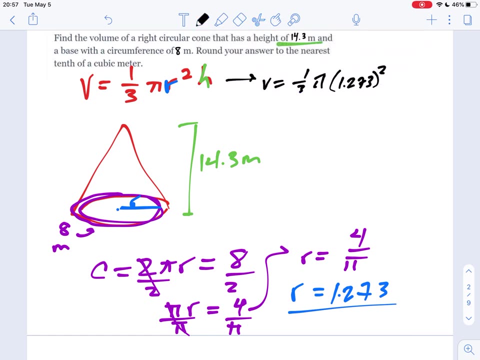 going to do is plug it into the formula. So the volume is equal to 1 third pi times the radius, which we just found squared times. can I fit it? Nope, Another crisis, averted Times the height. And the height has been sitting here the whole. 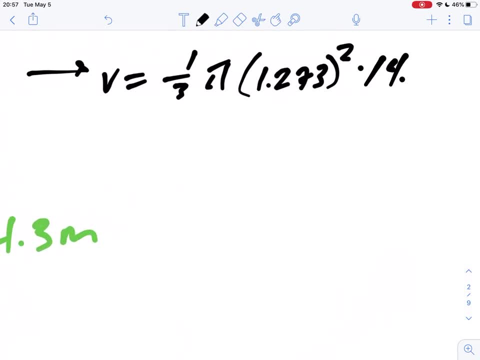 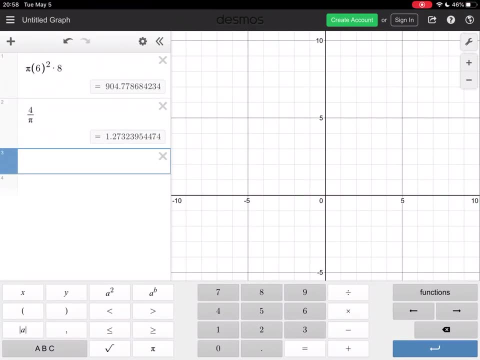 time: 14.3.. So let's see how my short-term memory works in remembering all these numbers. to type it in: 1 third: pi: radius: 1.273.. squared: 1.273.. squared pi: radius: 1.273.. squared pi radius 1.273.. squared. 1.273.. squared pi radius 1.273.. squared pi radius pi radius 1.273.. squared 1.273.. squared pi radius 1.273.. squared pi radius 1.273.. squared. 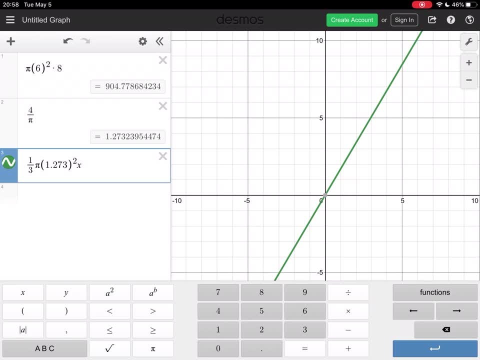 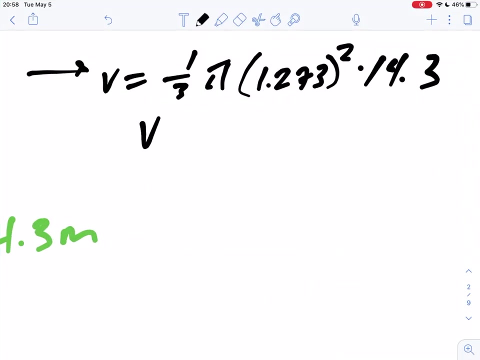 1.273.. 0.273,, 0.273,, 0.273.. dissect times the height and we get 24.267, so this simplifies to 24.267.. We have square meters and then meters, so this will total out into as volume always.